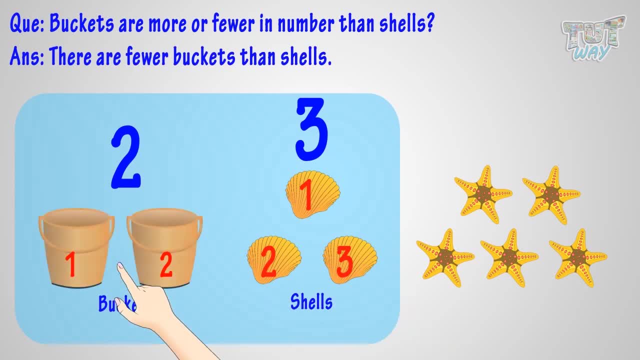 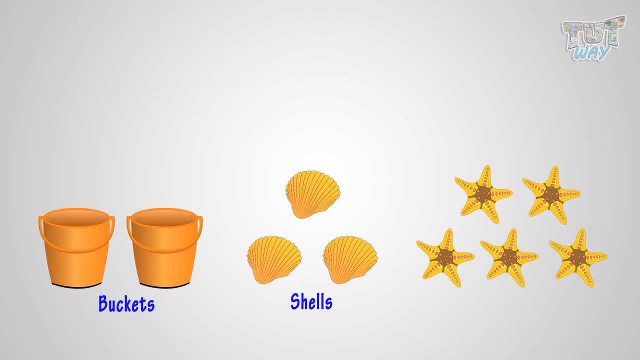 So there are fewer buckets than shells. Have a look at these things. Now tell me Starfish are more or fewer than shells. Let's count. One, two, three. Shells are three in number. One, two, three, four, five. Starfish are five in number. 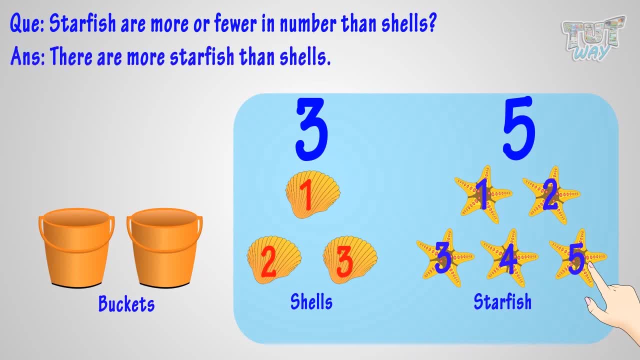 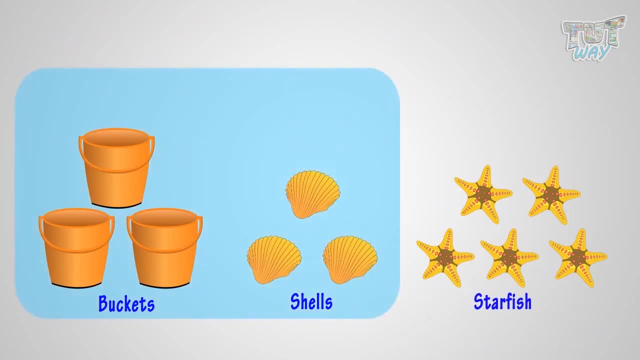 So there are fewer buckets than shells. Now tell me, Buckets are more or fewer than shells. So there are more starfish than shells. Now, if I add one more bucket, then there would be as many buckets as shells. See, 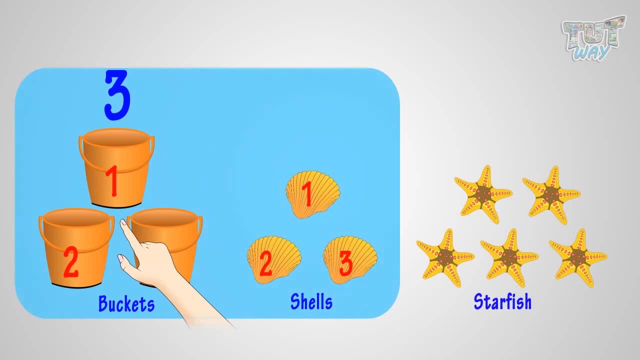 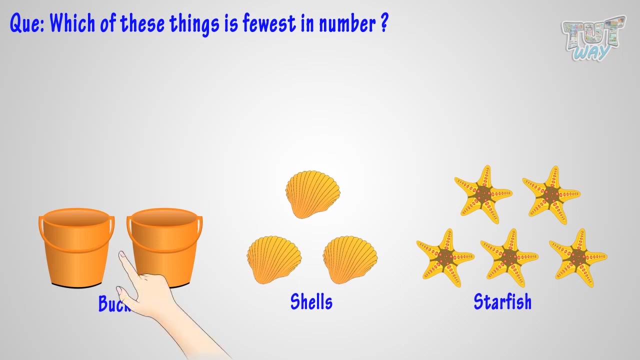 Buckets are three And shells are also three. Good, Now, which of these things is fewest in number? Yeah, Buckets are fewest in number, As buckets are two, shells are three and starfish are five. Hence, buckets are the fewest in number. Good, Now let's take another example. 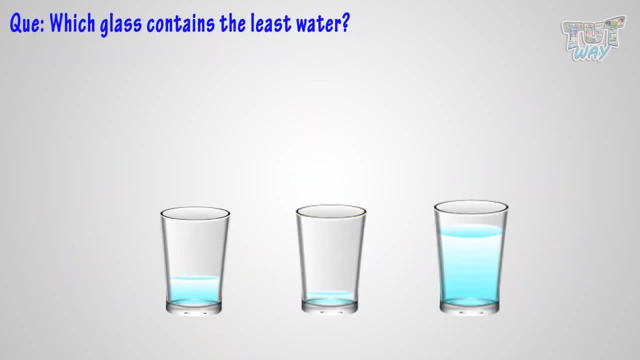 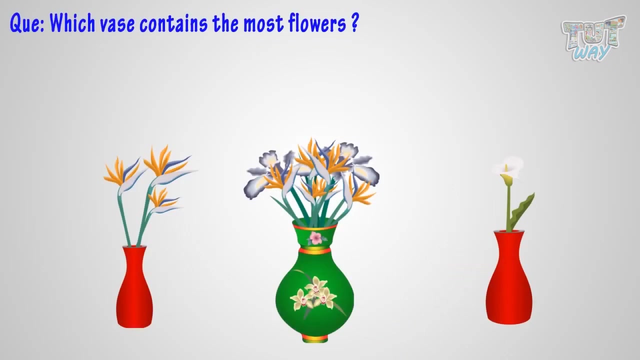 Which of the glass contains the least water? This glass, No. This glass, No. This glass, Yeah, This glass contains the least water. Good, Good, Let's take another example Now. which vase contains the most flowers? This one, No. 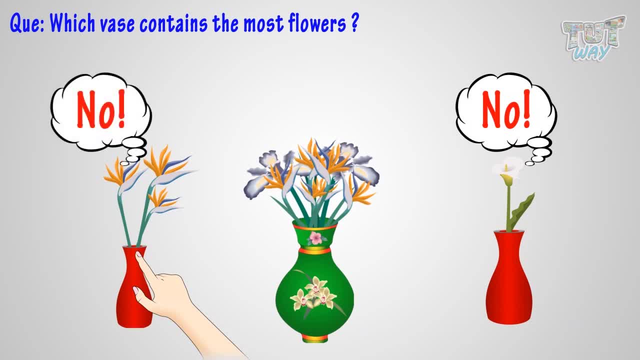 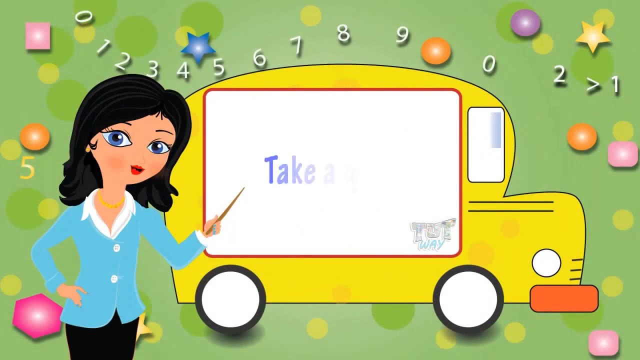 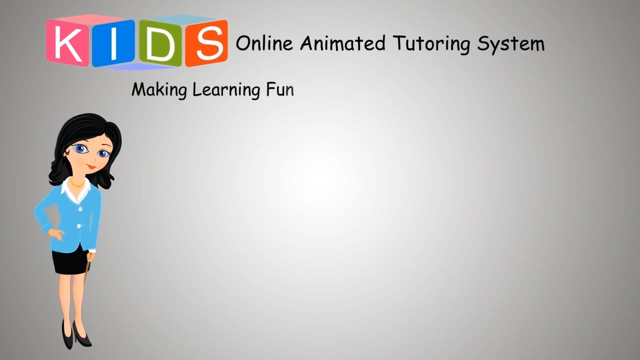 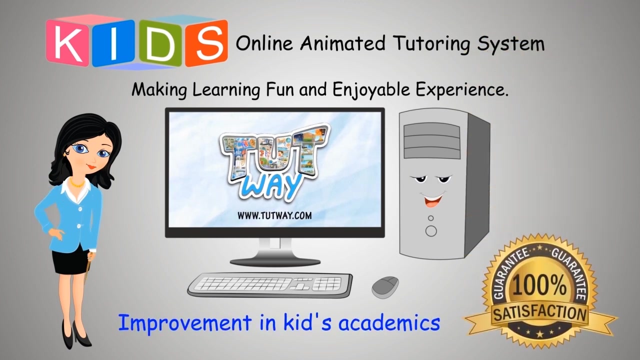 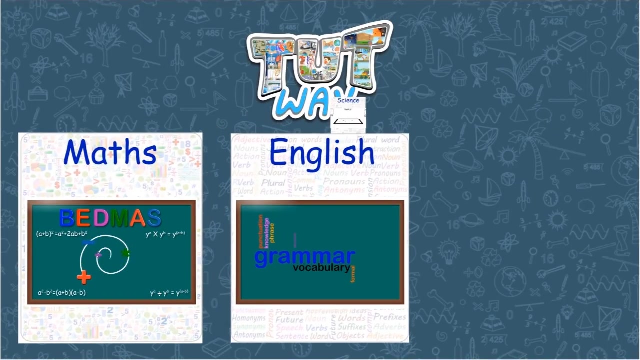 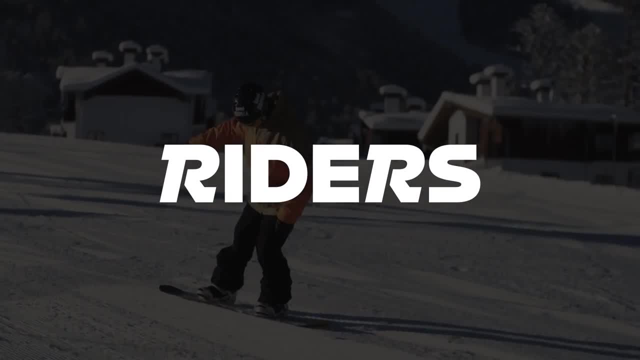 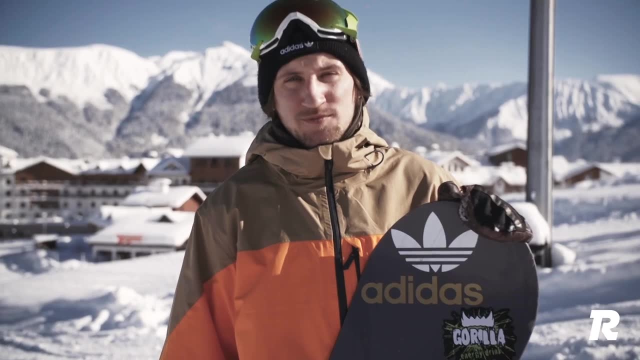 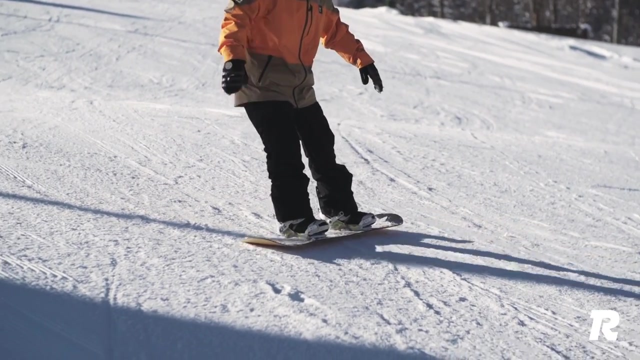 Hi guys, I'm Anton Lavrincev, and today I'll be teaching you how to ride the snowboard. If you've already gotten a feel for the heel edge and can control your speed and direction while riding on it, then it's time to move on to this next exercise. 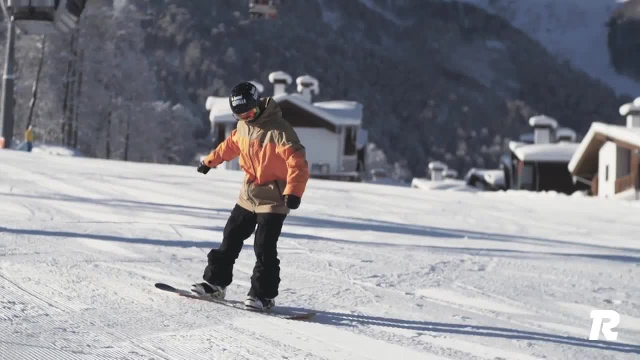 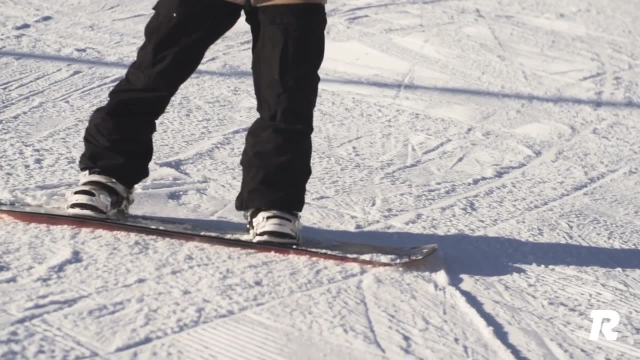 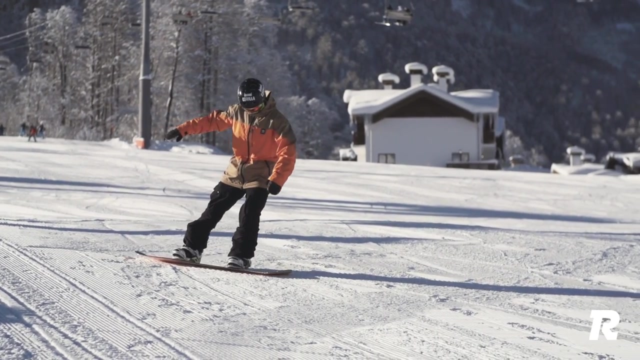 What you'll be trying to do is ride straight on a flat board and brake, controlling your speed. Start off with a heel slide. Now shift your weight onto your front foot. Your board will begin to move diagonally. Keep your eyes in the direction of movement. Continue holding. 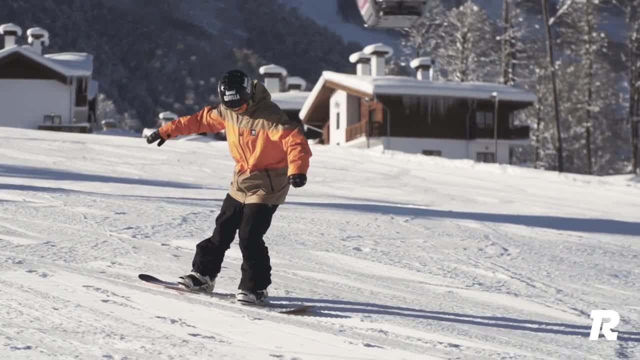 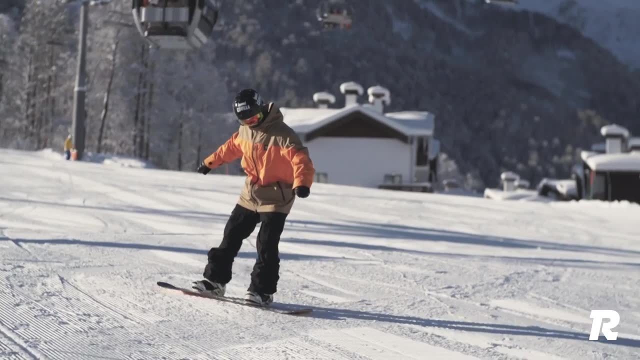 your weight over your front foot. Lower your toes, ending up on a flat board. This position will have you accelerating very quickly, so keep it short and shift your weight onto your heels. If you've kept your weight over your front foot, then the board will begin to carve. 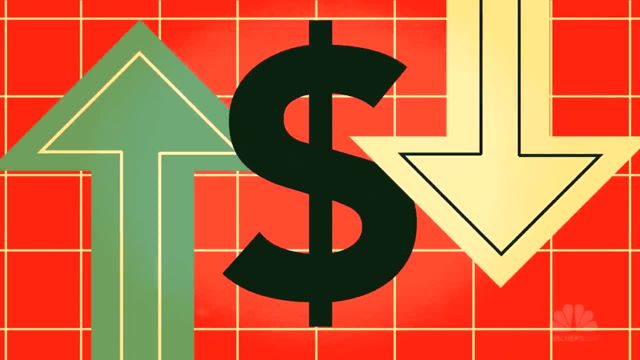 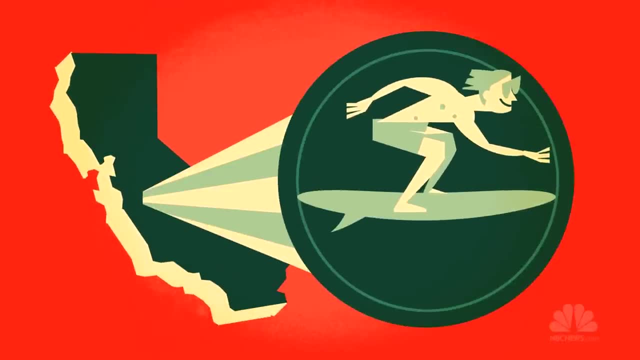 Let's say you're an economist trying to figure out if things in the US are getting more or less expensive. Well, you could look at the national averages, but that doesn't tell you the whole story. After all, over in California the price of surfboards might be skyrocketing. while in sunny Florida golf carts are selling for record low prices. Dentistry in Wisconsin could be pricier than ever, but you might get a good haircut in Seattle for under $10.. To measure how far a dollar will go, government bean counters, blend and weigh numbers.